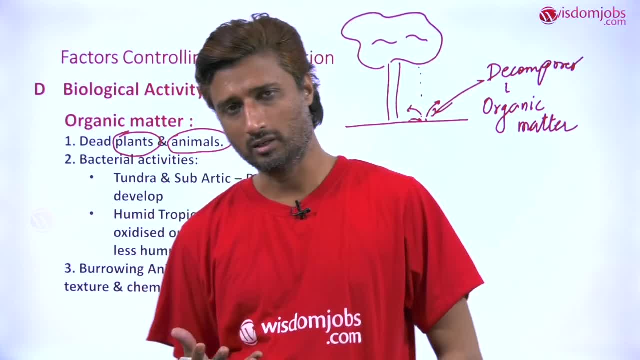 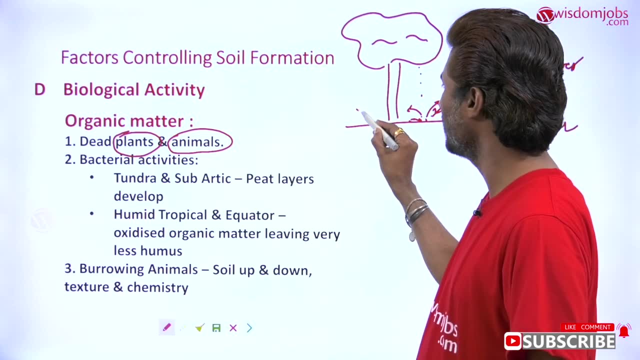 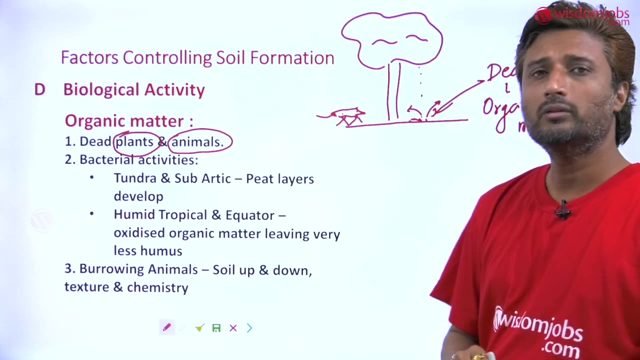 they all goes and decompose. So that is what organic matter. Okay, now this organic matter is released by means of the decomposition of leaves. in the similar way, if there is an animal dead body is there, it is also going to. if it is going to die, then the it. 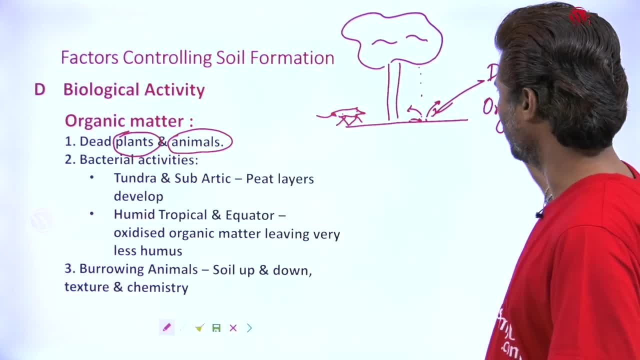 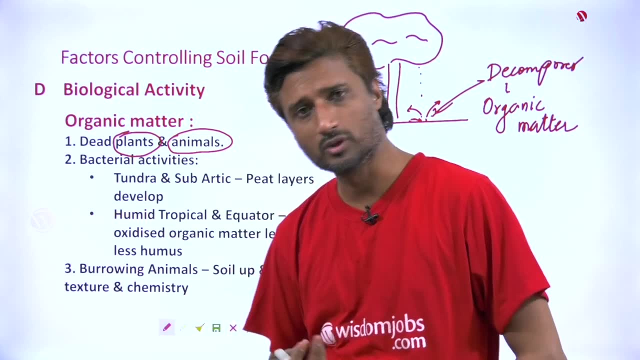 is. it is organic matter is going to roots by means of, again, The decomposer. Who are the decomposer? The bacteria or microorganisms, okay, and and other organisms, they act as a decomposer, Okay, that the next thing, that Y organic matter is important. 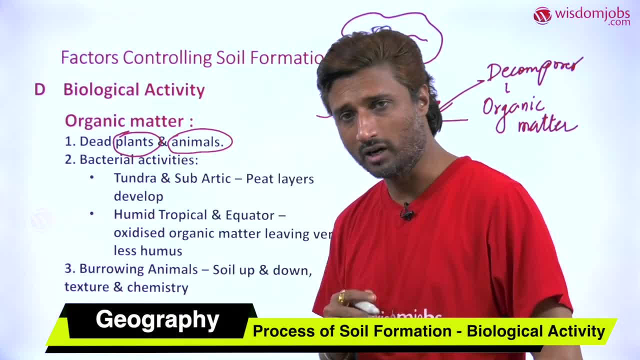 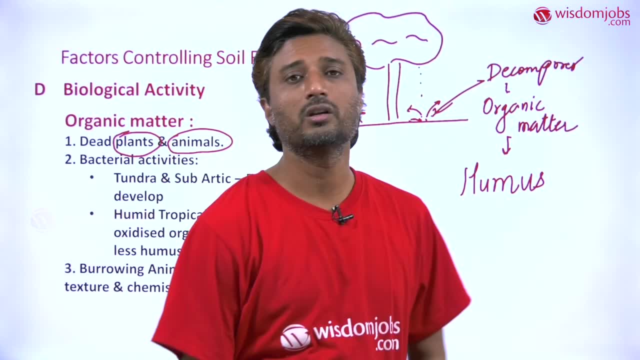 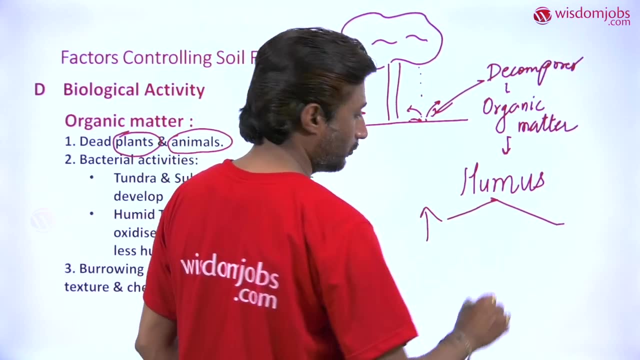 Let me you previously- you should have the concept why organic matter is important. This organic matter releases humus by means of humification. So humus is released by process of humification, then again depending on the proportion of humus, if the proportion of humus is high, 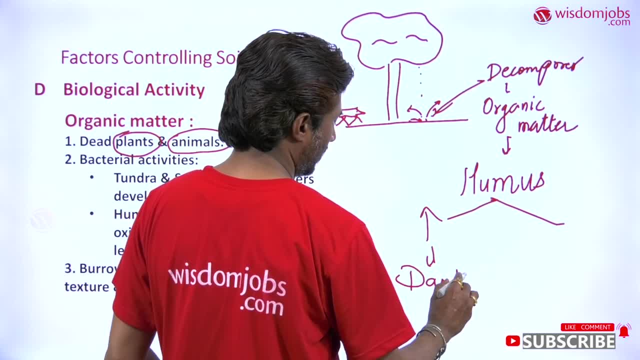 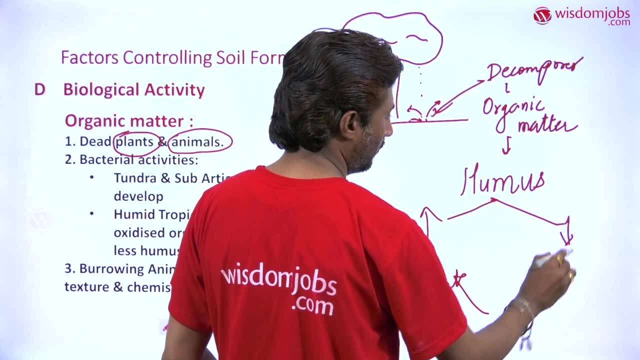 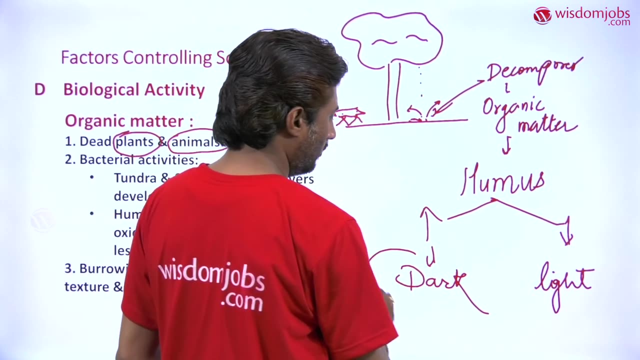 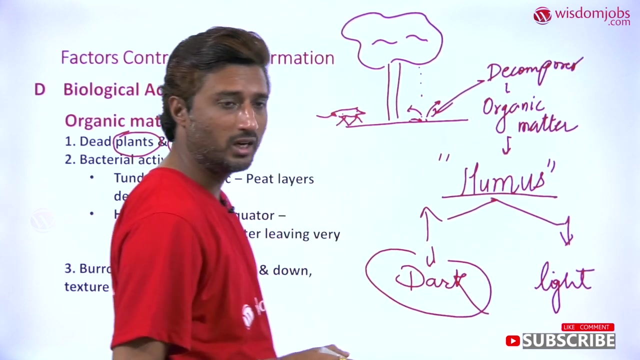 the soil will have somewhat dark color and it is said to be the fertile one. So the dark color soil will be fertile one. If the proportion of humus is low it will have light color. So the color of the soil again is decided by the proportion of humus and also its fertility. 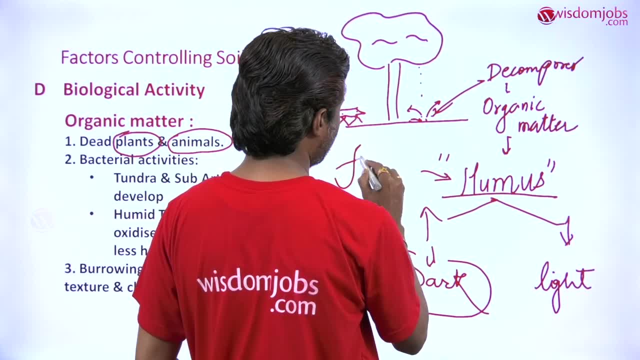 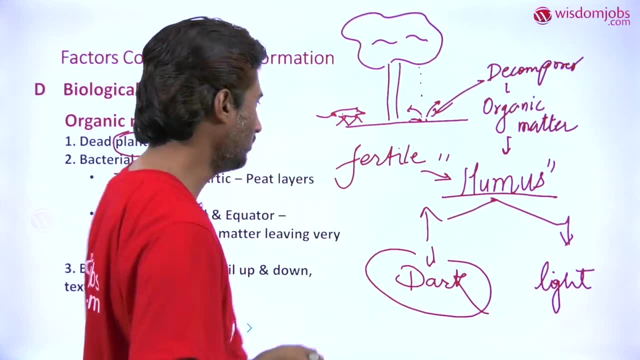 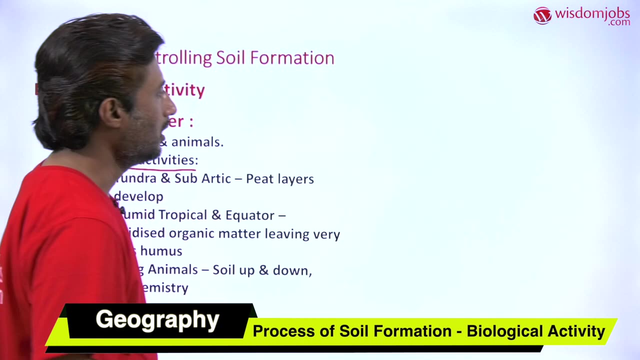 is decided The humus, decide more humus, more the soil is fertile, So more humus is there, more it will be fertile. Now, condition, condition, Now coming to the back, next point: the bacterial activities. So again, as I told you, on the soil, 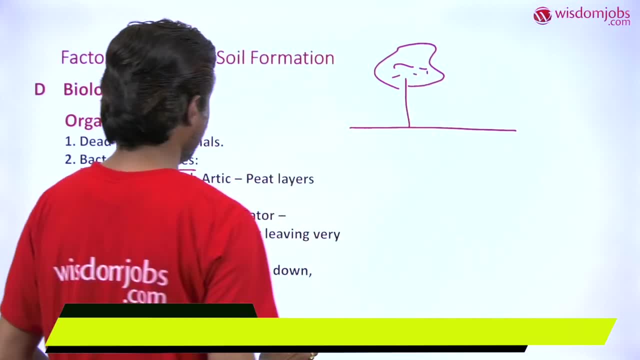 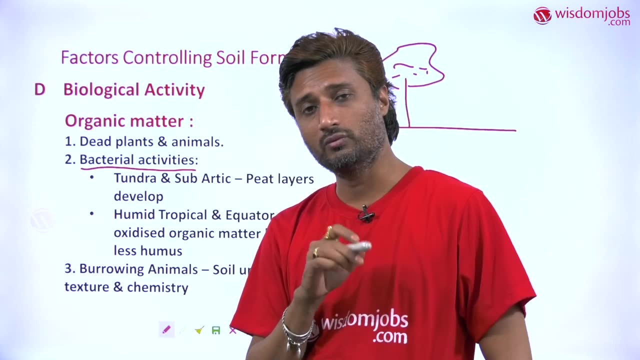 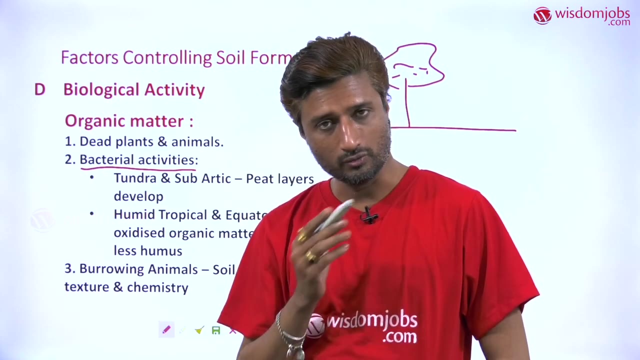 okay, the bacterial activity: what is actually doing? in my previous video also, I told you about the bacterial activities: how the temperature- it was in content with temperature, So how the temperature increase, the bacterial and chemical activity. If you have not gone through that video, please go through that video so that you should understand. 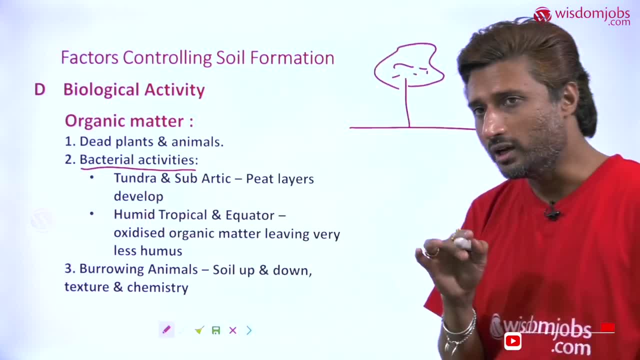 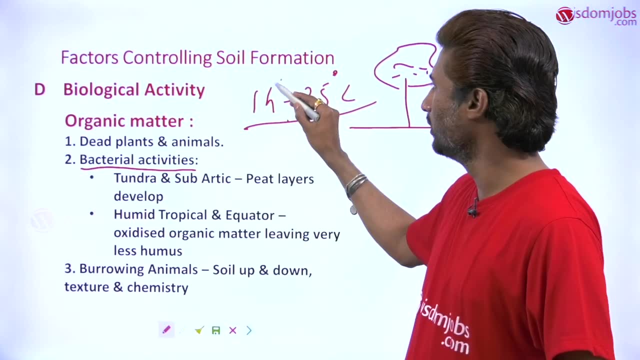 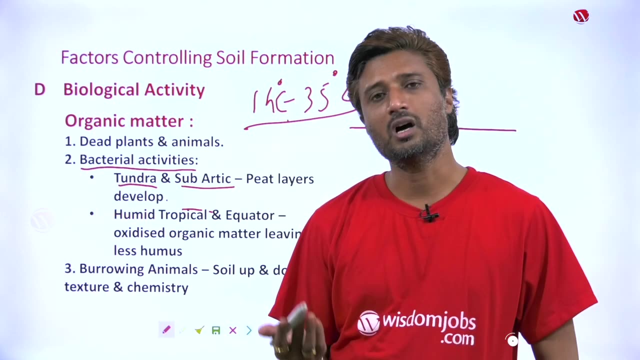 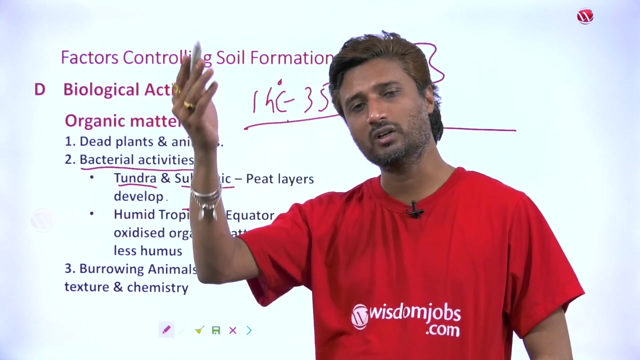 So if bacteria are present, So that this person comes in between. so in the sanitaryselsteral process of the humus, the soil structure is going to be more or less identical with the physical. Porque pos Men, is there a need for the sound of humus? yes, I had to remember this. 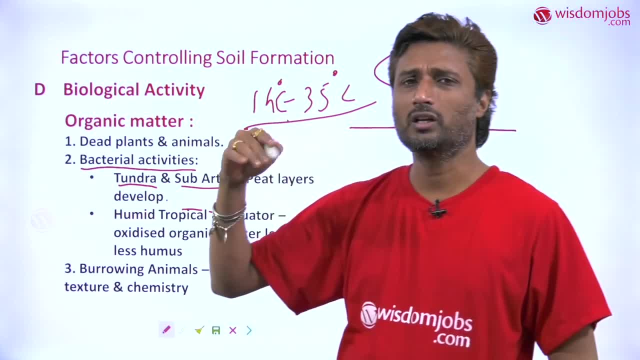 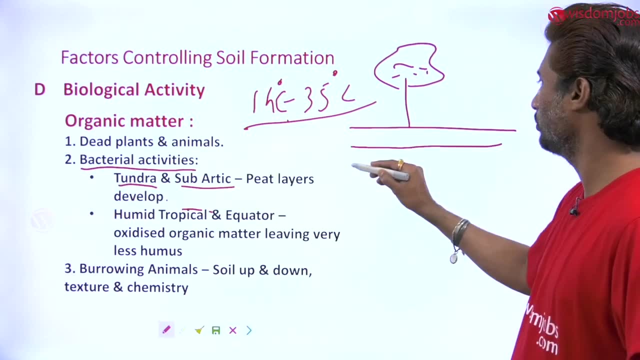 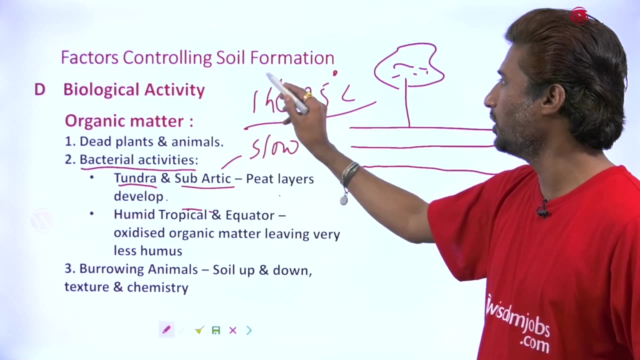 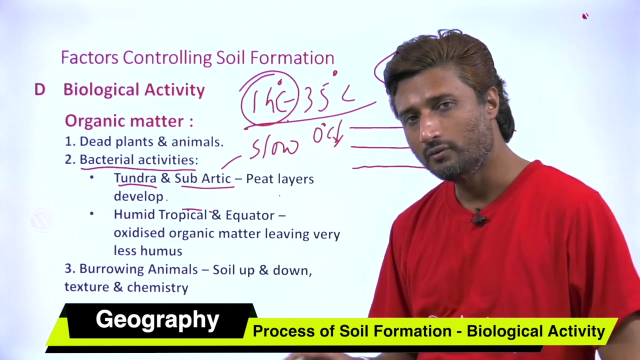 because I have it nonetheless. I have written the numbers above 50 degree north. So that region. here the bacterial activity will be slowed down. ok, So here the bacterial activity will be slowing. So here it is slow because the temperature is at freezing point below 0 degree Celsius, ok, or nearly freezing point, ok, So bacterial. 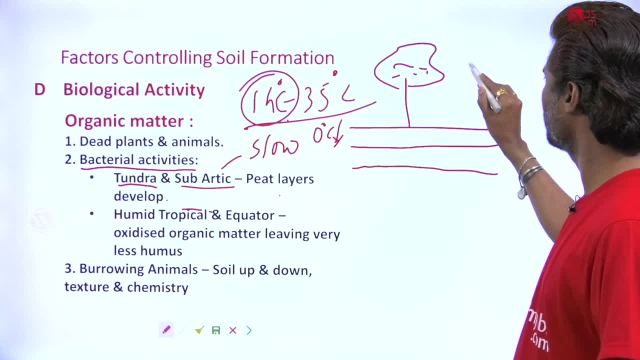 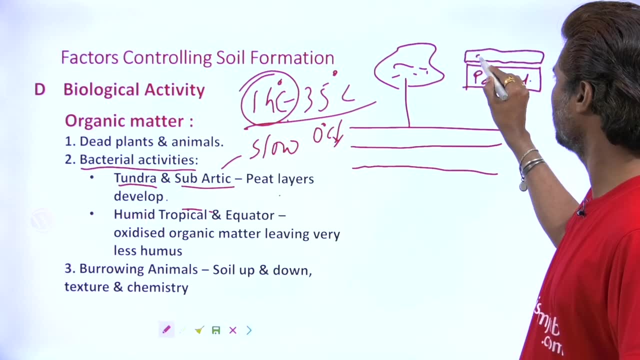 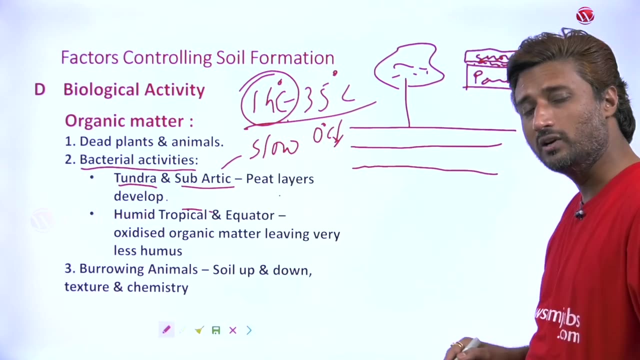 activity will be less. So in tundra region the condition will be like this: the parent rock material and over it the soil. sorry, the snow is there, So here very less chances of forming the soil, as the bacterial activity is very low. So this soil becomes young soil. 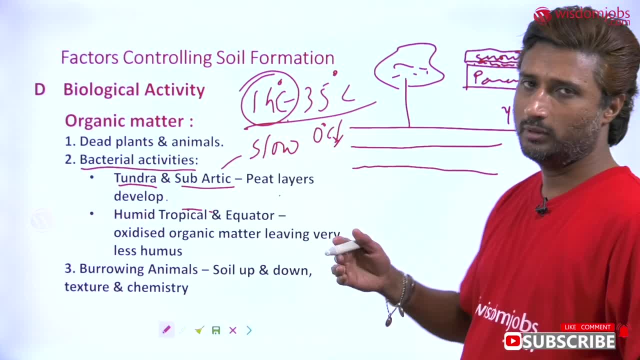 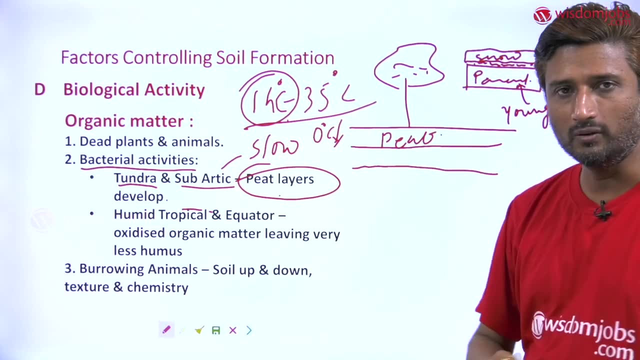 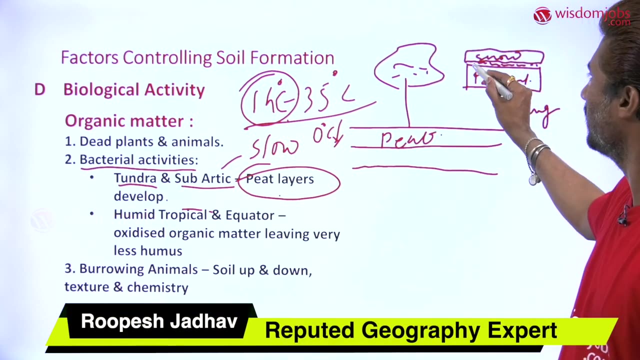 ok. So in sub arctic region it will be little bit layer. So here the peat layers are going to develop, So the various layer of peats are going to develop instead of soil profile. Soil profile is not developed there. So here, as you see, parent rock material and suddenly 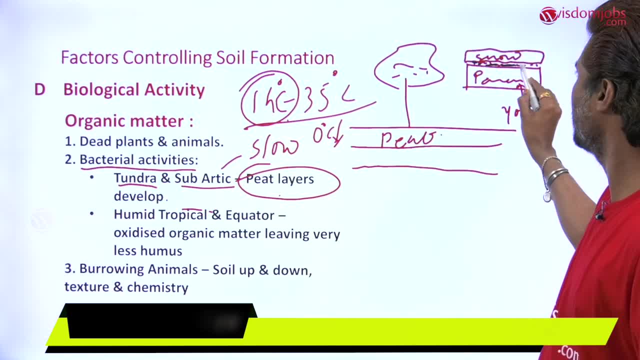 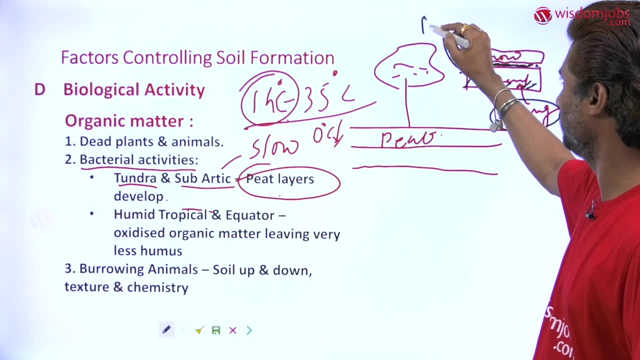 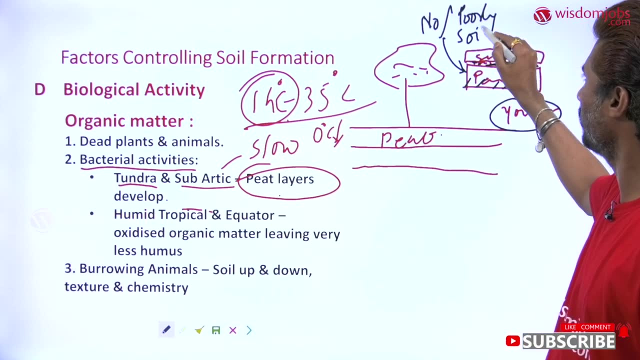 the soil part. ok, So here the soil is there and parent rock material beneath. So there will be no soil profile in tundra or arctic region, no soil profile or poorly develop soil profile. Poorly develop soil profile- ok, So here the peat layers are going to form, So 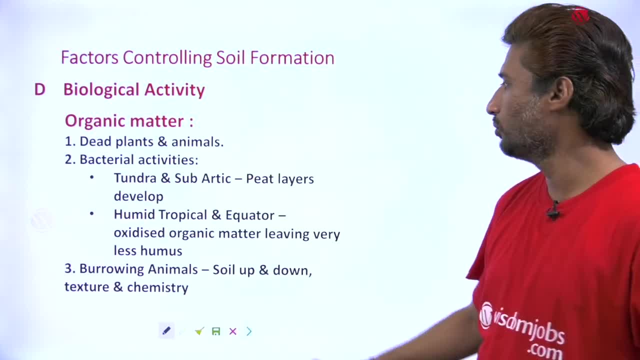 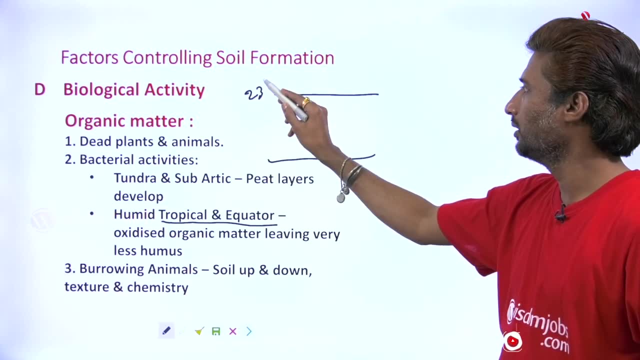 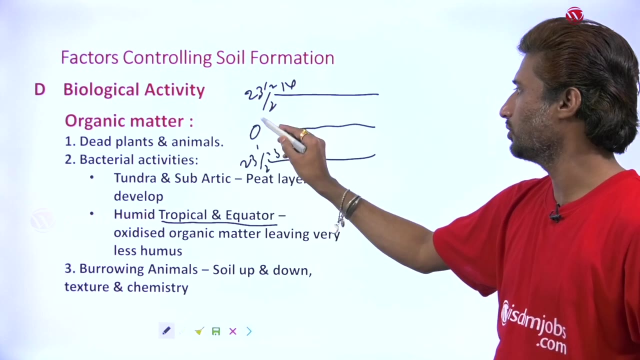 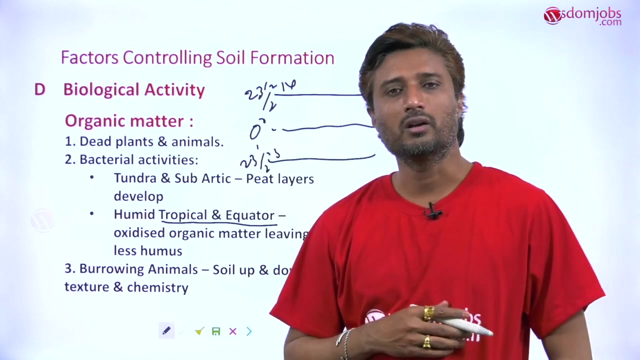 Then now coming to the next region that is humid, humid and tropical equatorial region. so you might be knowing, this is the tropic 23.5 degree north and 23.5 degree south and in between there there is equator 0 degree. this is that region. equator is that region which receives daily rainfall between 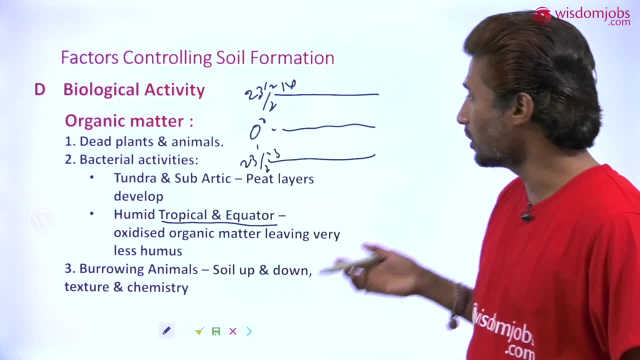 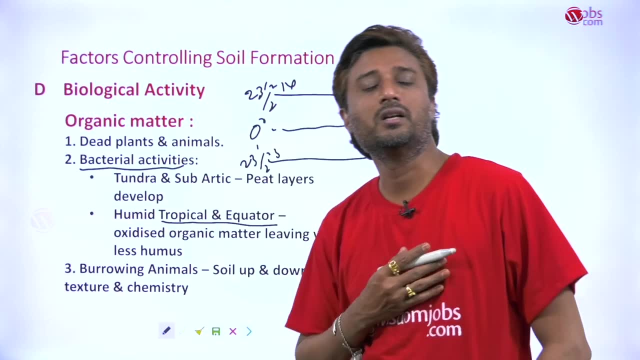 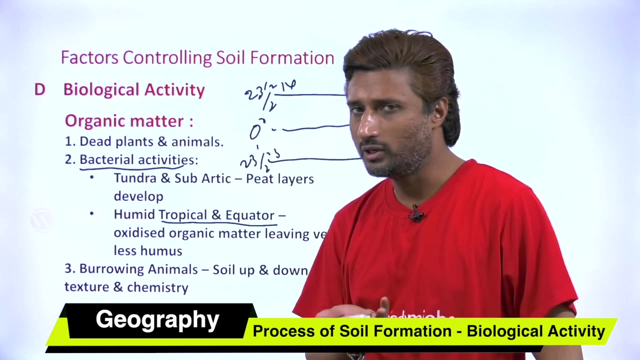 2 pm to 4 pm and abundant amount of sunshine, so which is a good place for develop, for the bacterial activities and also we. the India lies in tropical country and tropical monsoon type of climate, so we also. this part also receives the good amount of rainfall and sunshine. so here in 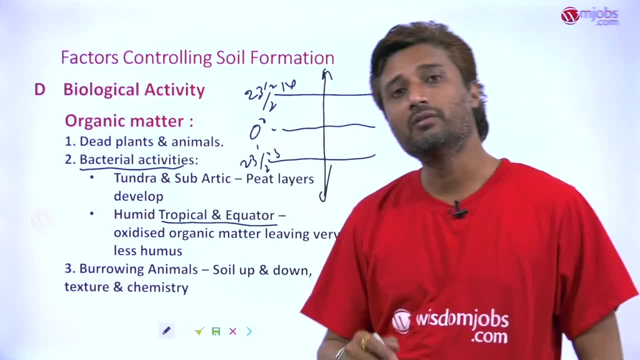 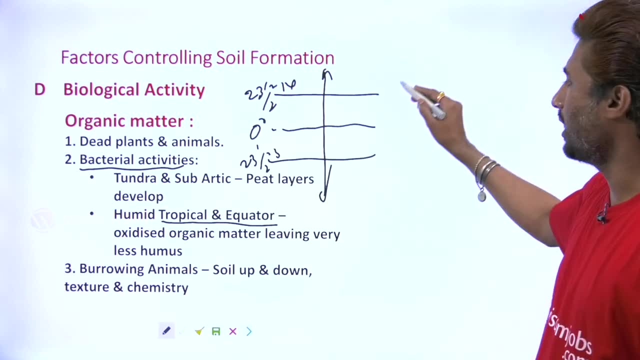 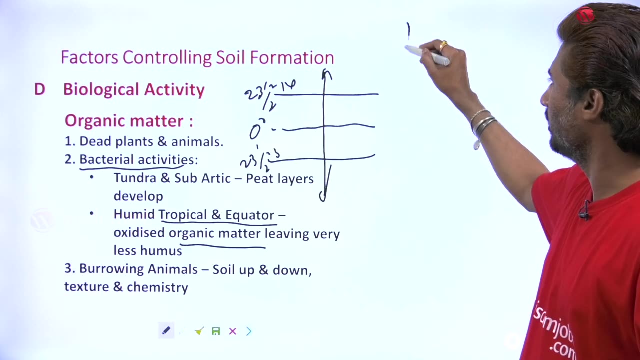 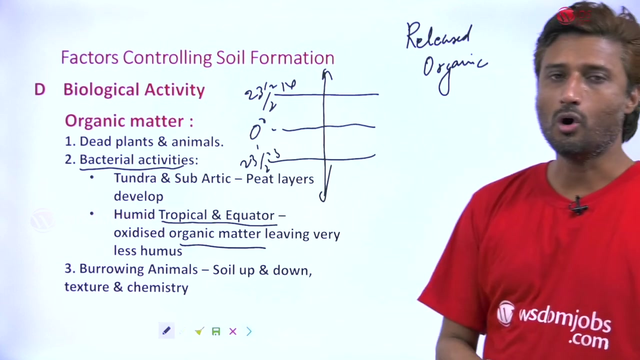 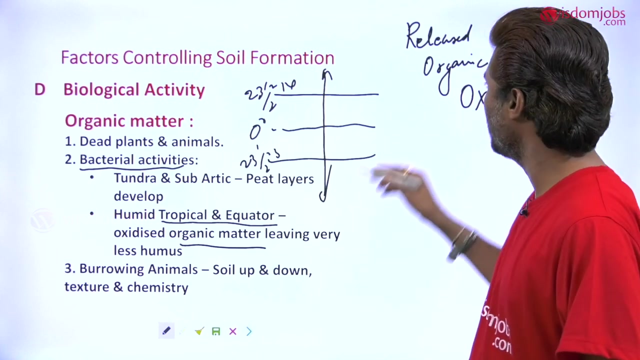 this region, the bacterial activity will be at higher level as compared to the tundra region, okay, or arctic region. so, but what happened here? as the bacterial activity is too high, it releases the organic matter. the organic matter is released, okay, so, release of organic matter, but due to oxidation or oxidizing process, okay, whatever the humus is. 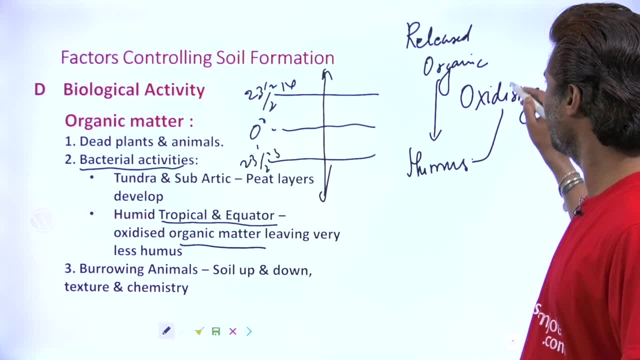 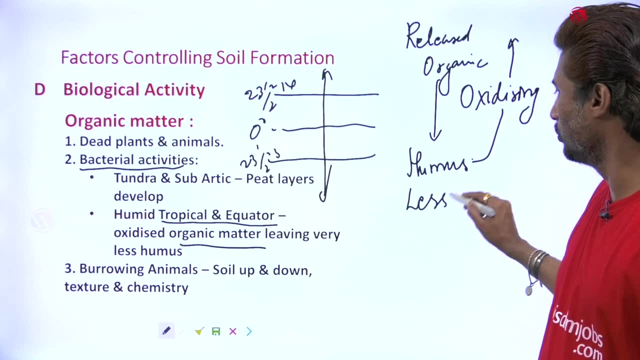 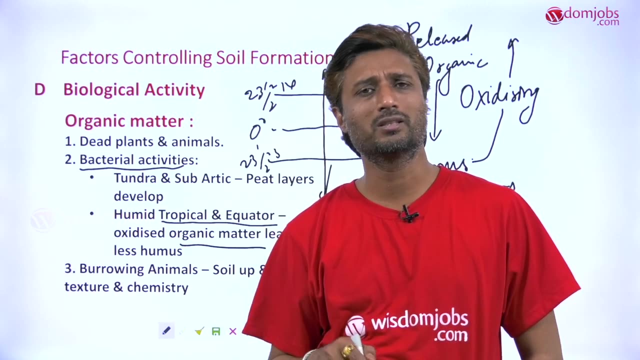 released that humus is evaporated. okay, that is loss. so here there will be less humus and in tundra region, as it is not getting completely decomposed, so the humus will be less there. so in temperate region, the process, the of your formation of humus. 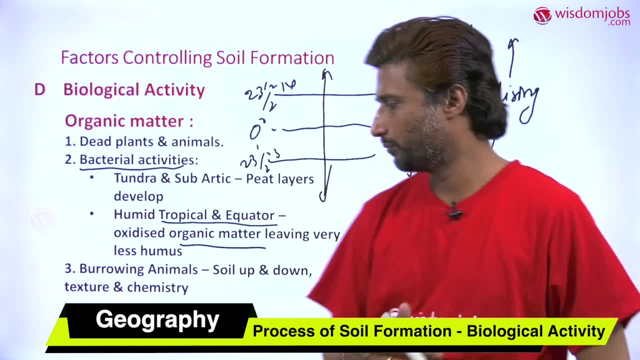 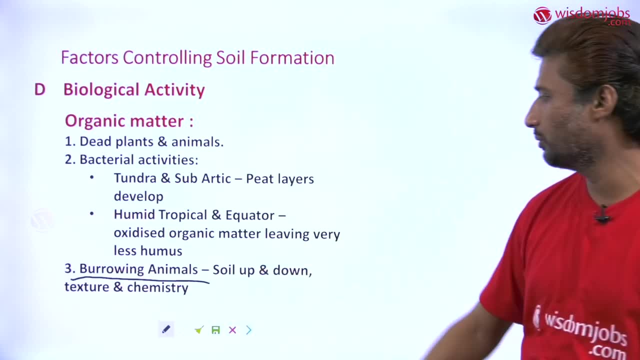 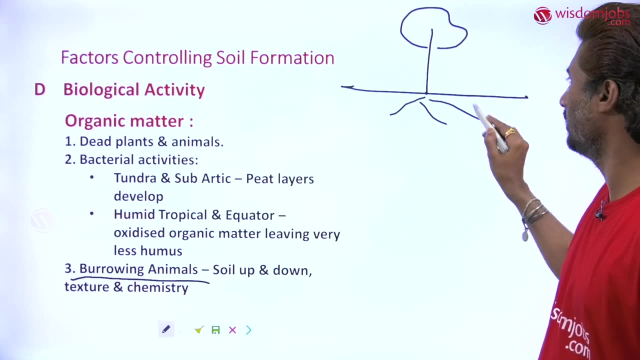 will be proper in proper way. okay, so this is going to happen in tropical and humid region. now the third one is the burrowing animal. what? how does the burrowing animal works? okay. so working the roots means it is very difficult for fauna to support the further living medium. 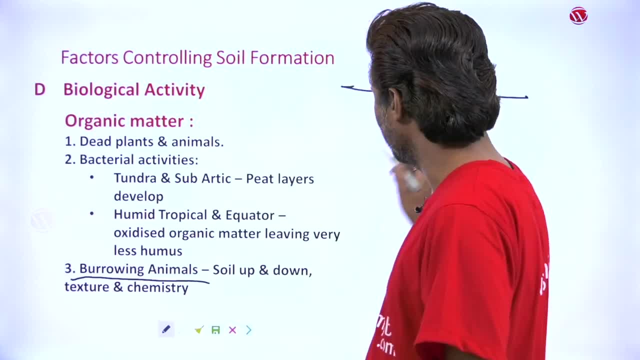 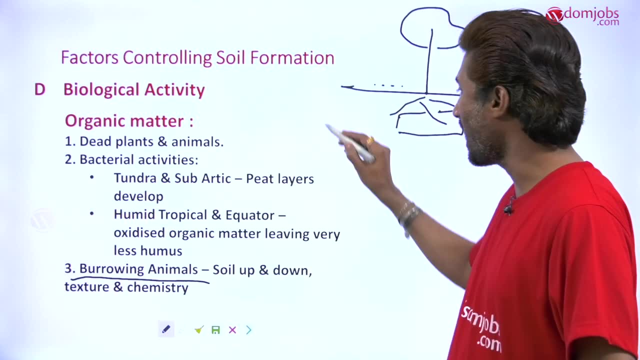 its uses is very difficult and it is also sometimes thatappeals to credit. it is not questão para bridging, it is the form of balancing theory of labour. alright, so if you am a farmer, you might say that if you are feeding yields like still, as I have told you. so these are the plant roots. they will hold the parent rock material. apply the pressure- physical pressure, mechanical pressure- and 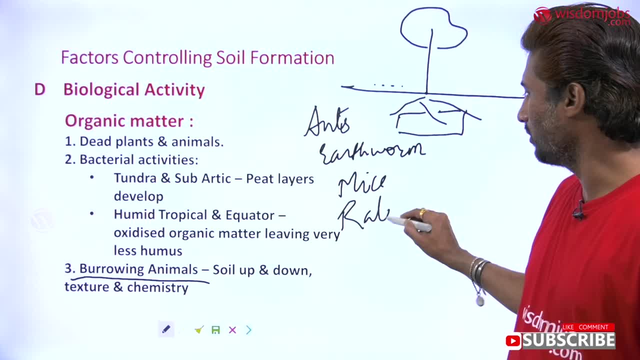 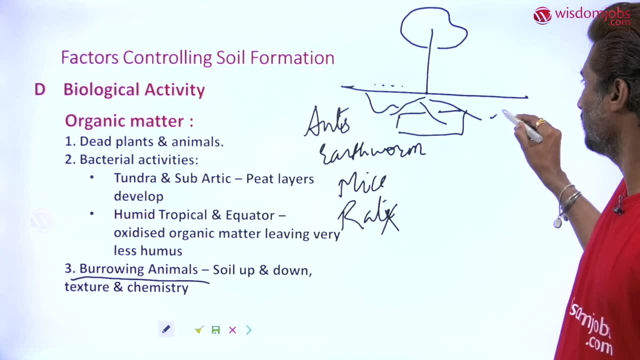 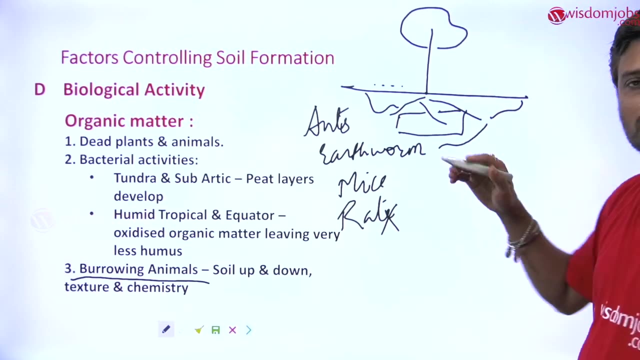 yes, if you have a vehicle, you must think how to work this, to get it going. it is very difficult. rat, okay, rabbit, what they do, okay. so they burrow the ground, okay the layer, to the deeper extent. they eat, for example, rat, they eat the rock part, they erode the rock part by means of biting it. 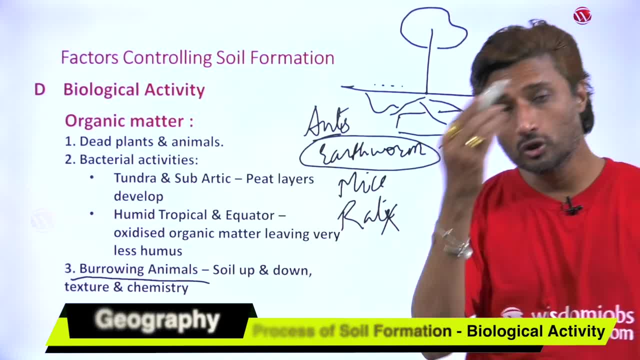 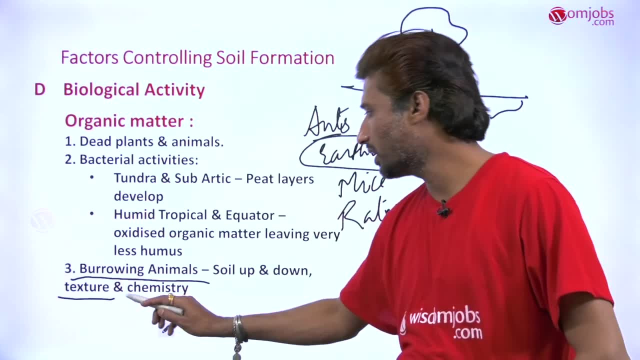 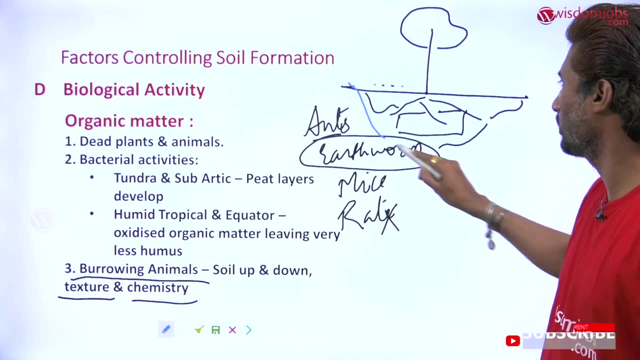 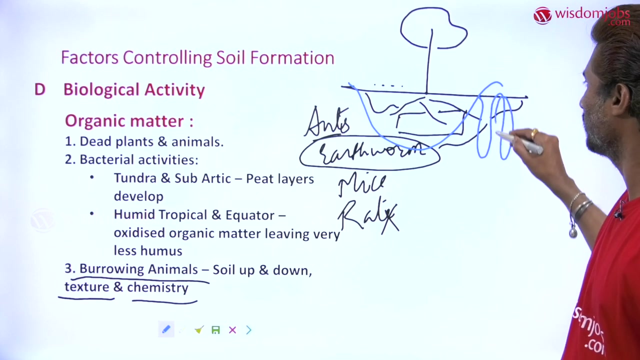 okay, earthworm, you might be knowing, it consumes the soil and then it leave behind. so this all changes the texture, structure and the chemistry of the soil, also, while going down and coming back. okay, so it makes the soil movement up and down. okay, so, going down, coming up, going down, coming up. 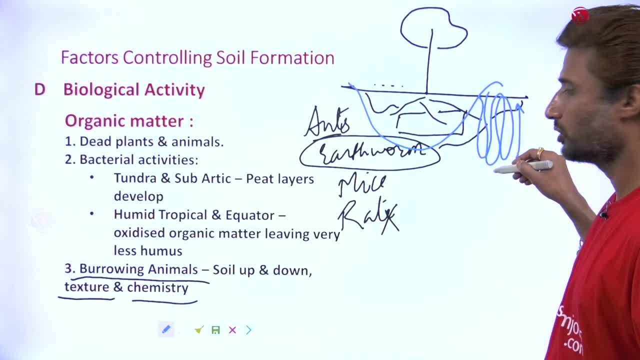 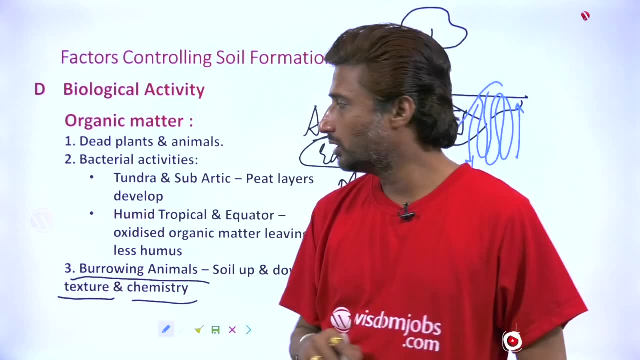 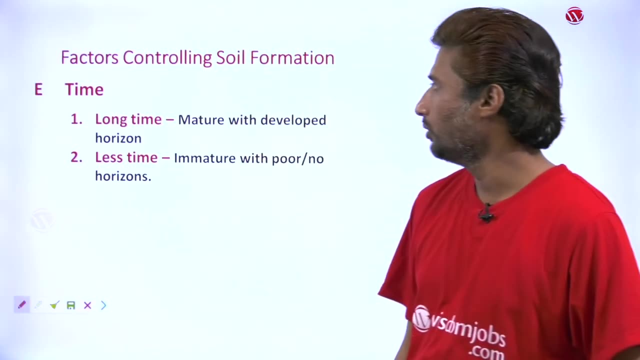 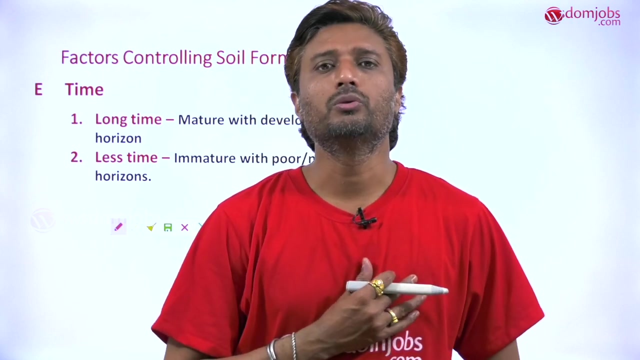 so this: the soil head from the lower layer is deposited upper part and upper layer is taken to the lower layer. okay, so this is what all about the biological activity. now, next part: the time factor. okay, so how the time factor is affecting the formation of soil. now, friends, let me tell you. 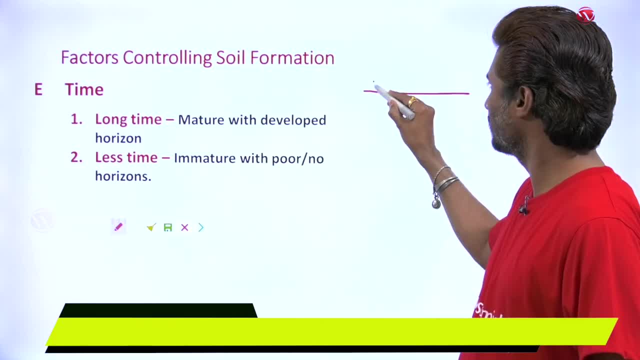 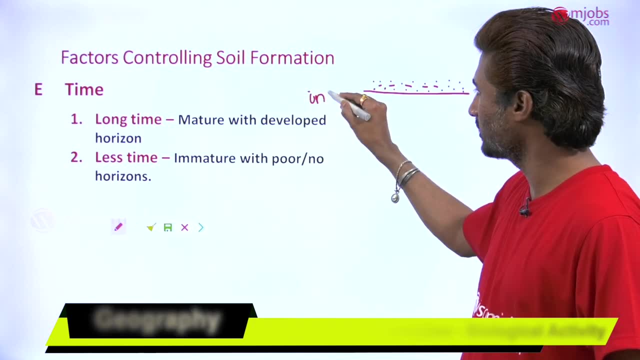 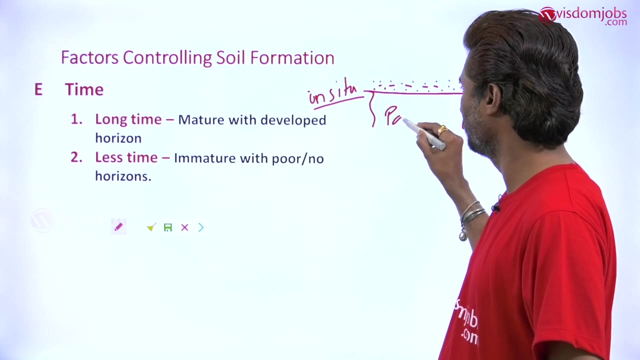 if this is the parent rock material and this is what soil deposited over it or formed over it, okay. if it is formed in situ, at the same place, okay, in situ, that is weathering of this parent rock material and the soil is remaining at the same point, okay, so what? 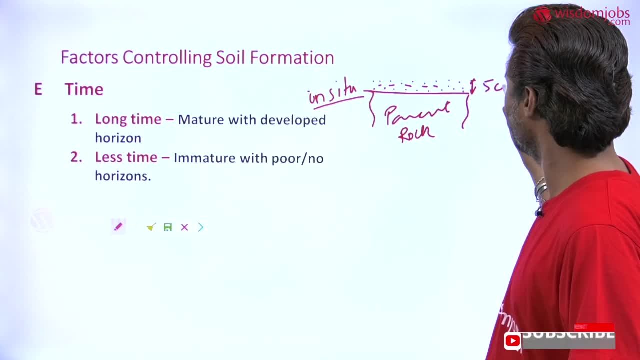 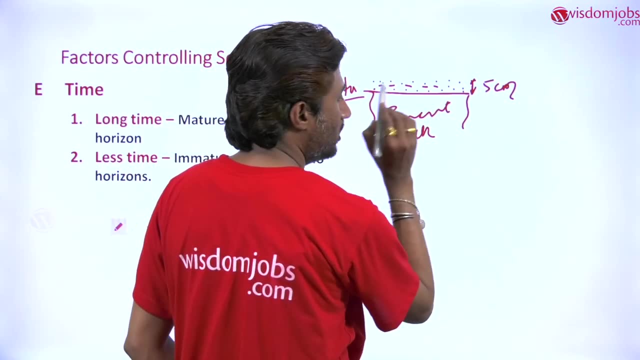 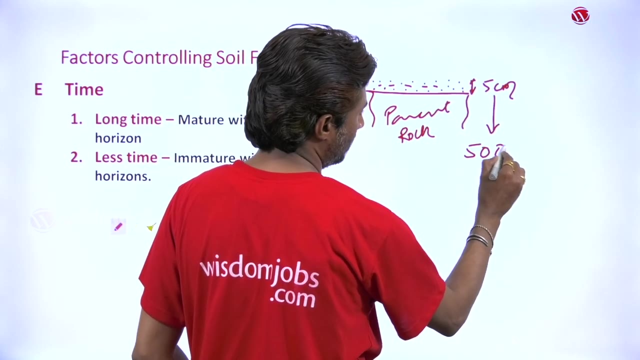 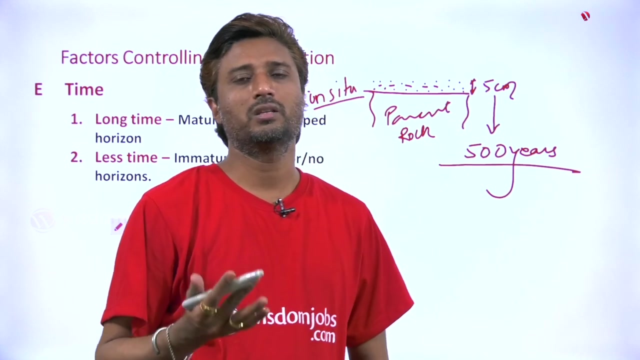 if the thickness of this soil is of five centimeter, will you believe that the formation of the soil for the five centimeter, if it is totally undisturbed, nothing human activity or interference is there. it talks near about 500 years, so the time span close hell is very much important in this context. we say that africa continent is. 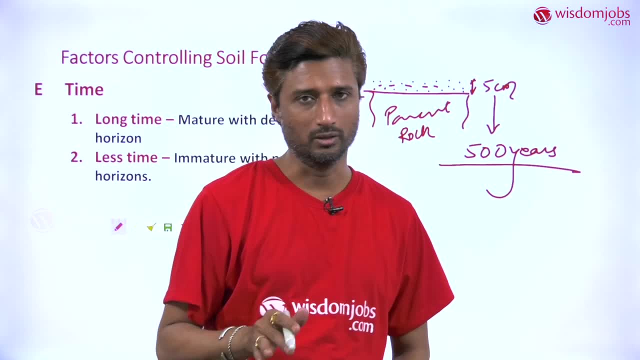 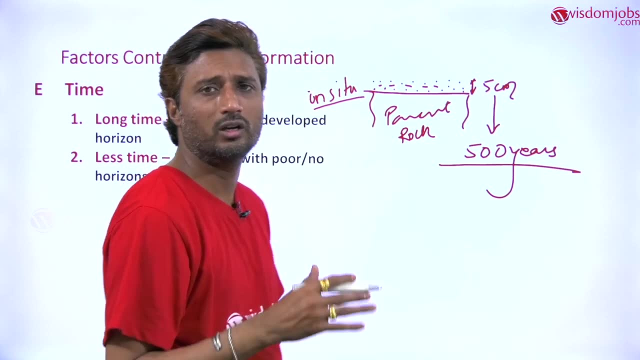 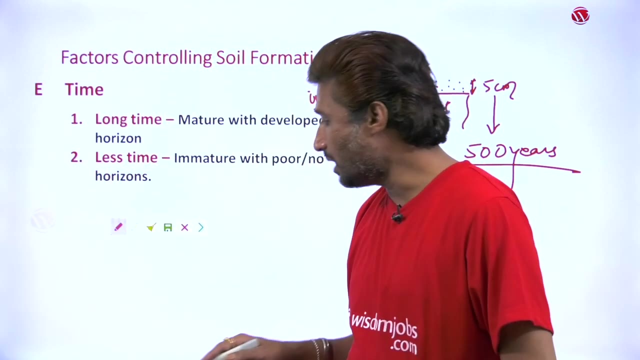 a virgin continent. virgin means untouched, undisturbed. okay, so to form the soil of five centimeter, it takes 500 years. and africa is that continent in which there was no human interference, no disturbance by human being. okay, so again, if i am talking about the time duration, 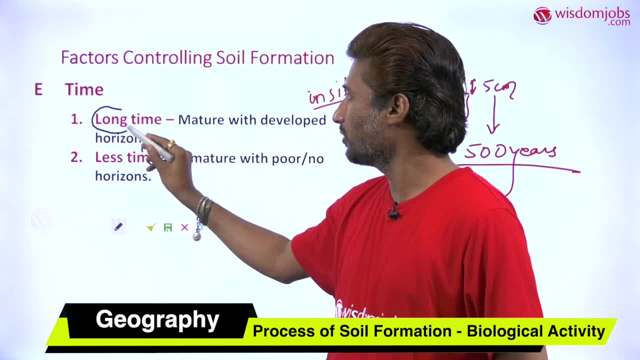 so one more thing is that if it is going to take sufficiently long time, the mature type of soil is göreburredburnt- see again if i am talking about the time duration. so one more thing is that if it is going to take sufficiently long time, the mature type of soil is going to win over, provide continuous growth space. soil is developed Again. the soil with matured soil means it will have soil horizon. The soil horizon will develop in sufficiently long time. If it is taking less time, then immatured or young soil is developed with poor or no horizons. But all these both means. 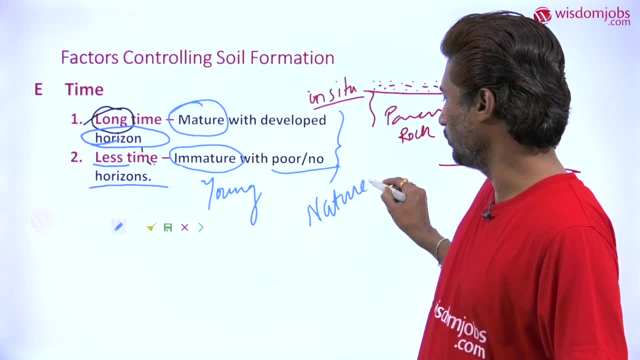 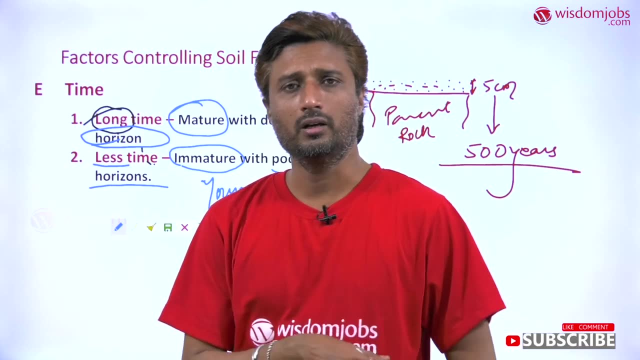 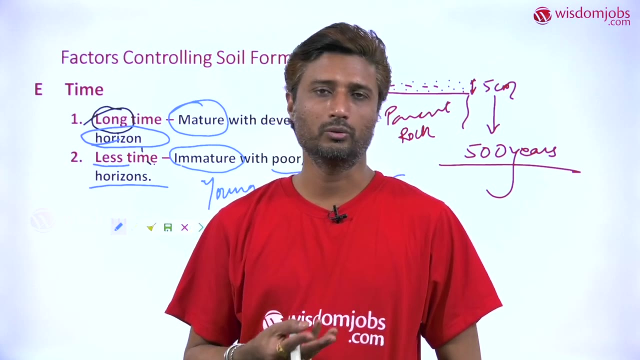 with the by nature. only If human being is entering in that part with the help of the heavy machinery, within a day it can break the rock, which took at least thousand years on its own to disintegrate and decay, or due to the weathering process. So it is by means. 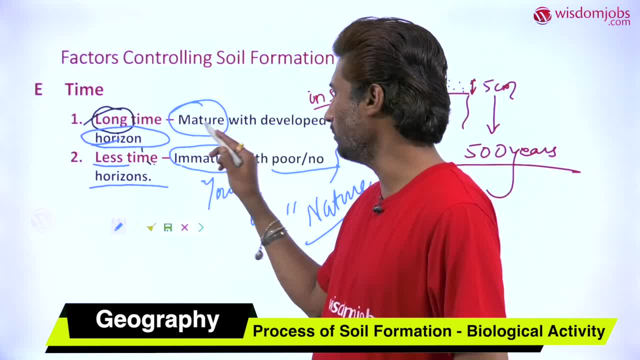 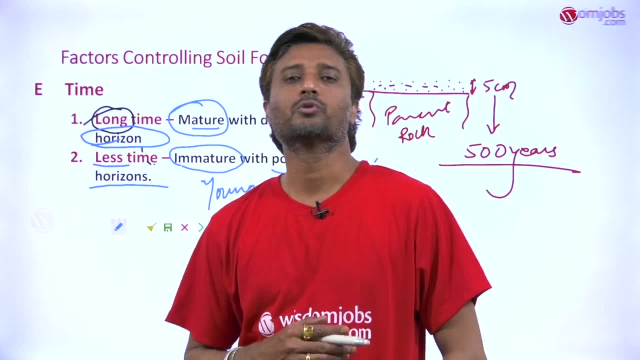 of nature. it will take sufficiently long time It is going to form matured soil with developed horizon. If it is taking less time, it will be immatured, with poor or no horizons. So this was all about the process of soil formation. So I think you might understood and please.